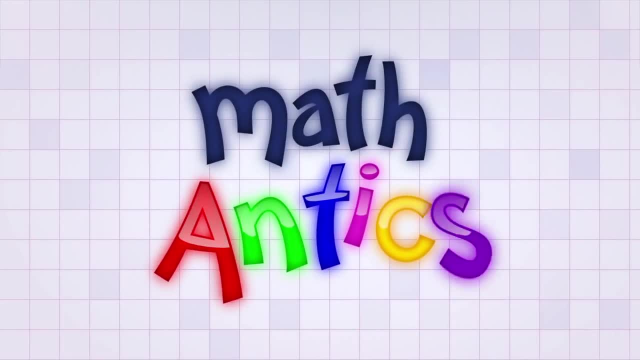 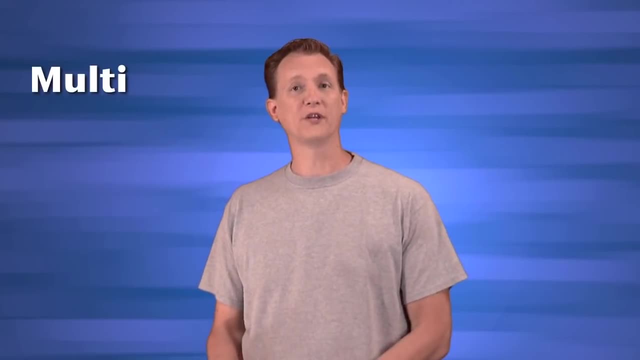 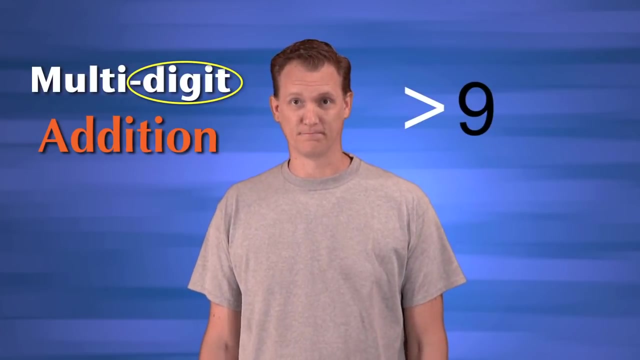 Hi and welcome to Math Antics. In this video we're going to learn how to do Multi-Digit Addition. A multi-digit number is just a number with more than one digit, which is anything greater than 9.. Two-digit numbers use two number places, like the number 32.. It has 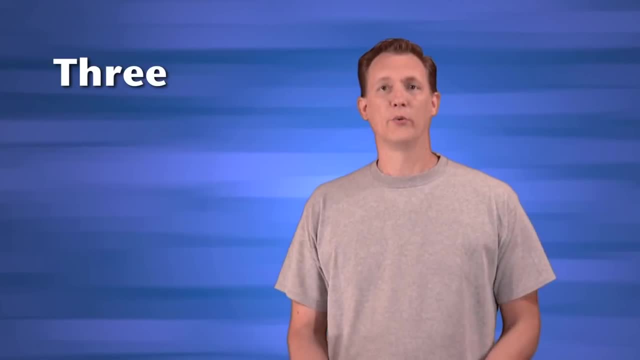 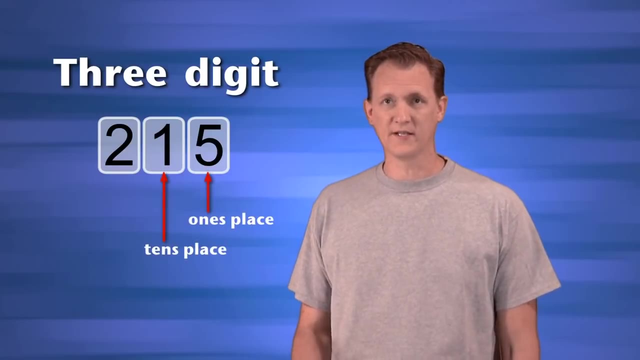 a 2 in the ones place and a 3 in the tens place. Three-digit numbers use three number places, for example 215.. There's a 5 in the ones place, a 1 in the tens place and a 2 in the hundreds place. But no matter how many digits a number has if you know your. 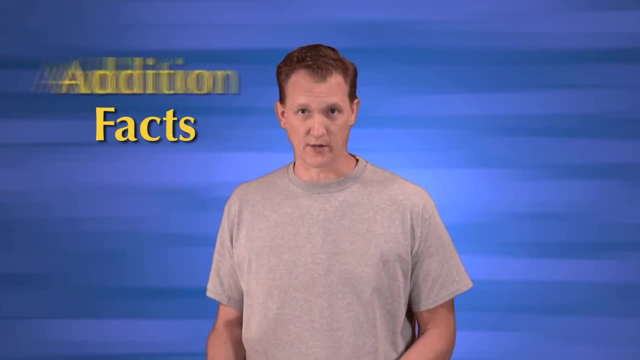 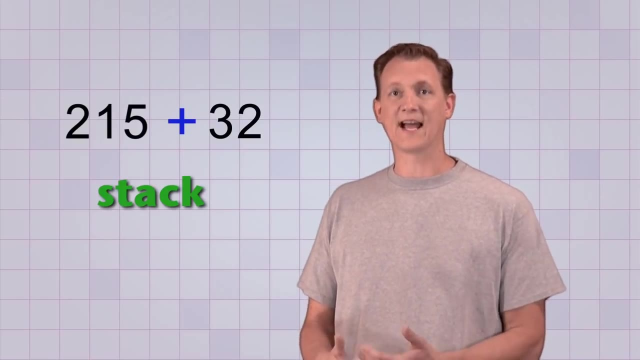 basic addition facts. you can add it to any other multi-digit number easily, So let's start by adding these two numbers together. Here's how it works. The first thing we need to do is stack the numbers up, And by that I mean rewriting them, so they're on. 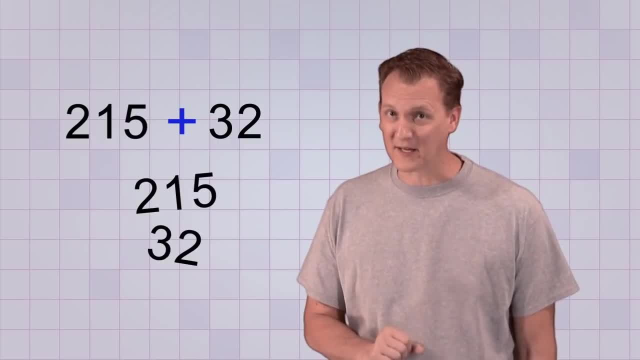 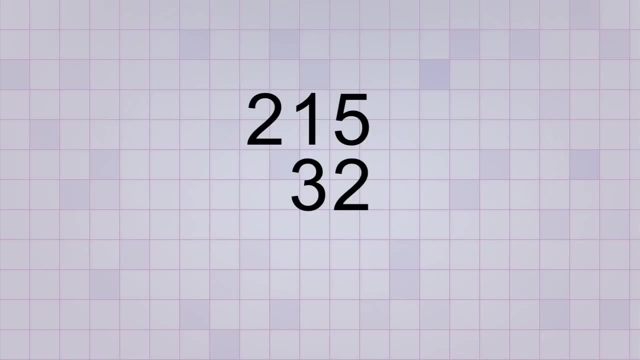 top of each other like this: Ah ah ah, Don't be sloppy. Make sure they line up nice and straight. That's more like it. But here's the most important part: Be sure to line up the number places so that they're. 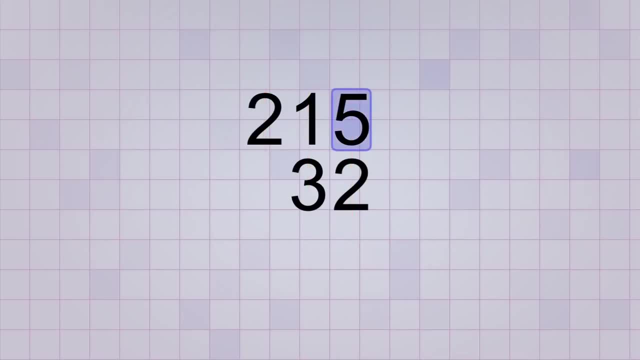 directly over each other, So that the ones place of the number on top is directly over the ones place of the number beneath it. And if you line up the ones place correctly, then all the other number places will be lined up too. The tens place are also lined up. 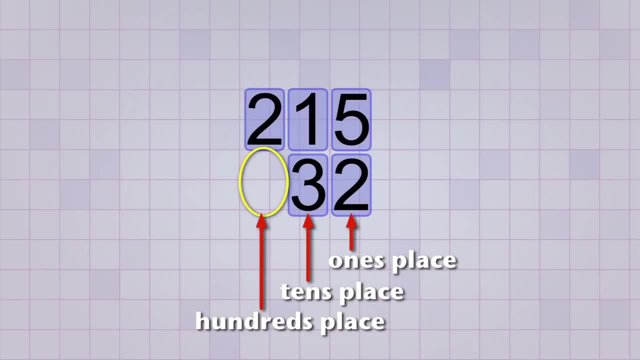 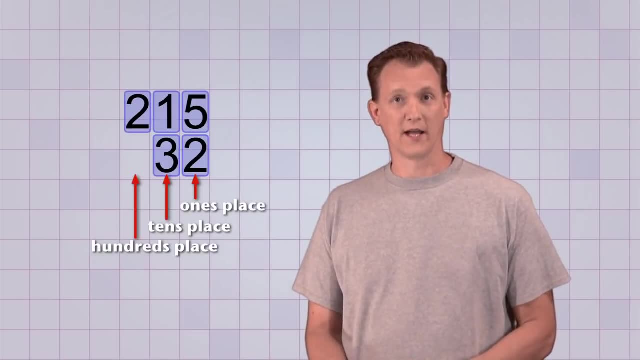 And the hundreds places. Well, the bottom number doesn't have a digit in the hundreds place, but that's okay. We can just imagine a zero there as a placeholder. But we don't have to show it After our numbers are lined up. we draw a line just below the bottom number because 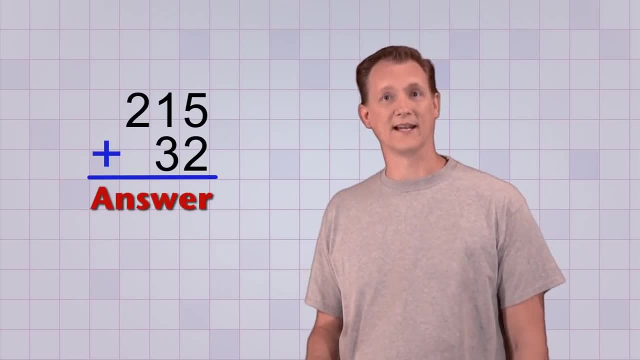 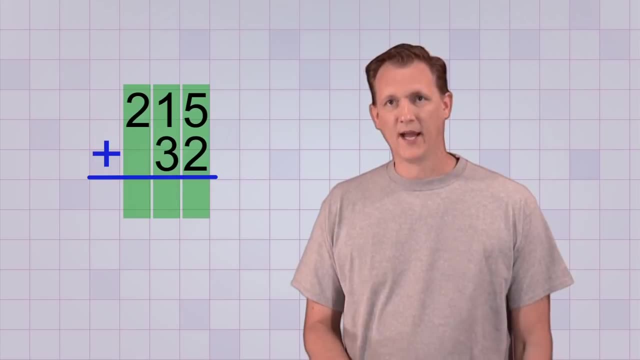 our answer is going to go below that. We also put a plus sign down here on the left side to show that we're adding By stacking the numbers up. we've formed columns for each number place and we're going to add the digits in each column. 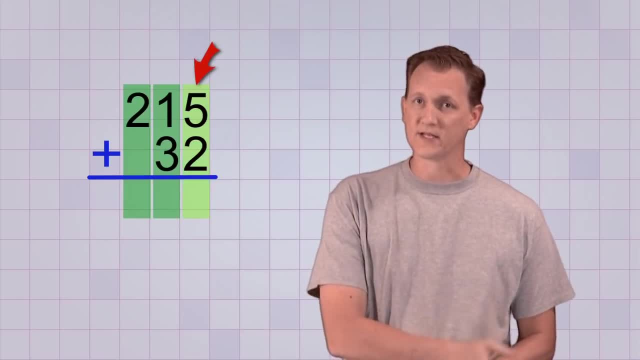 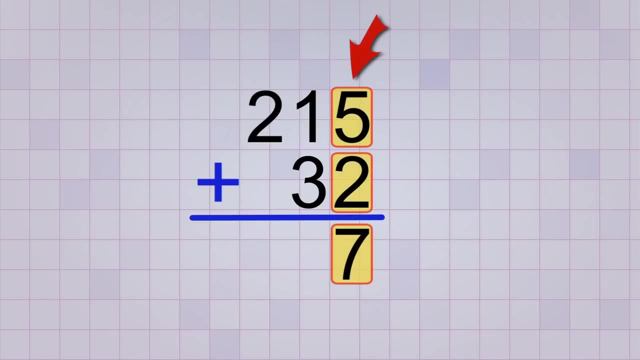 And this is super important. We always start with the ones place column and then work our way to the left, And in the ones place we have five plus two, which equals seven. So we put a seven in the ones place of our answer, which is just below the line. 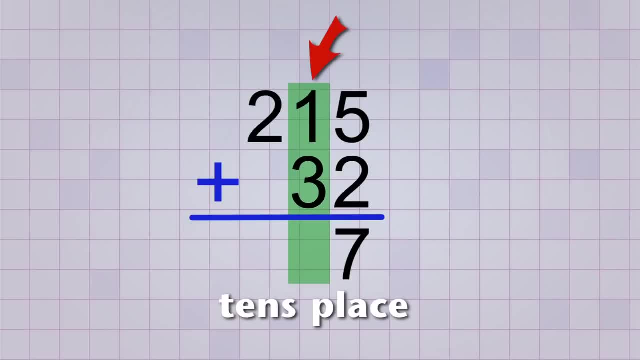 Now we can move left to the next number place column, which is the tens place, The digits: there are a one plus a three and that gives us a four in the tens place of our answer. And last of all we add the hundreds place column, But there's only one digit there. 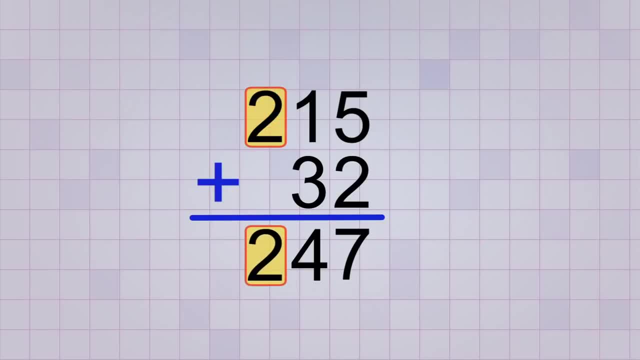 so we don't really have to add it. We just bring the two down to our answer like this. Of course, we could add the two to the zero that we imagined there as a placeholder, but zero plus two will just give us two also. 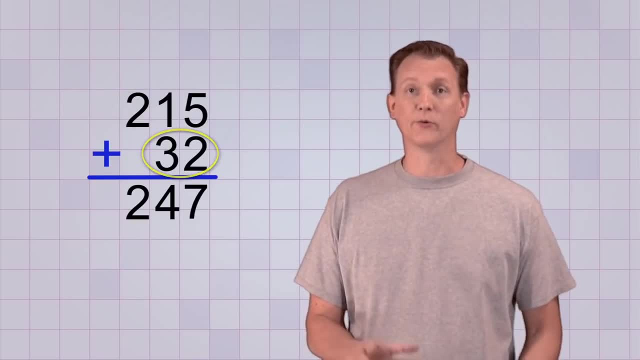 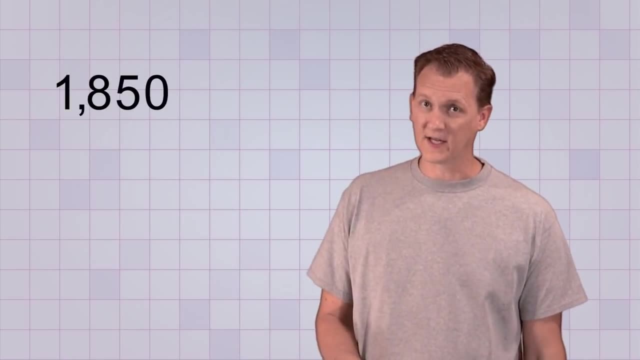 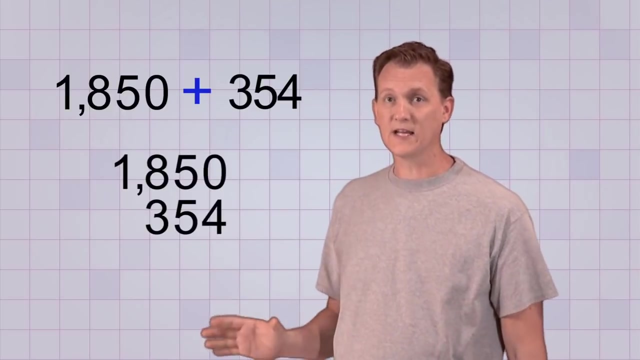 There, Two hundred fifteen plus thirty-two equals two hundred forty-seven. Let's try another example. This one's a little harder: One thousand eight hundred and fifty plus three hundred and fifty-four. Okay, the first step is the same. We need to stack the numbers up so we can add each. 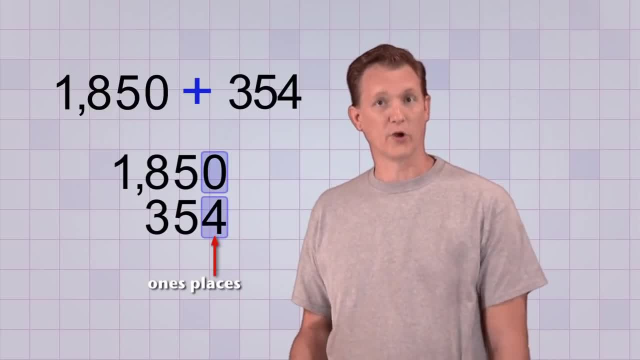 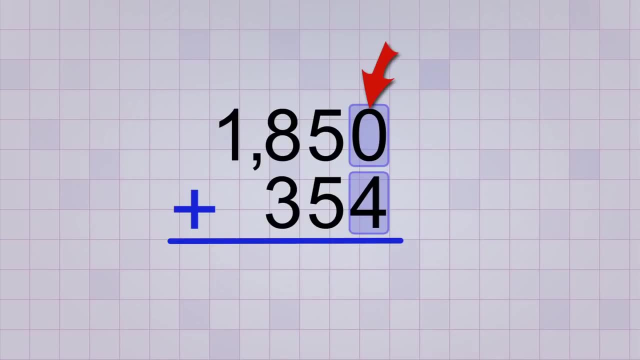 number place column. Be sure to line up the ones places and draw your line and plus symbol, just like in the last example. Again, we always start by adding the digits in the ones place. Zero plus four equals four, So a four goes in the ones place of our answer. 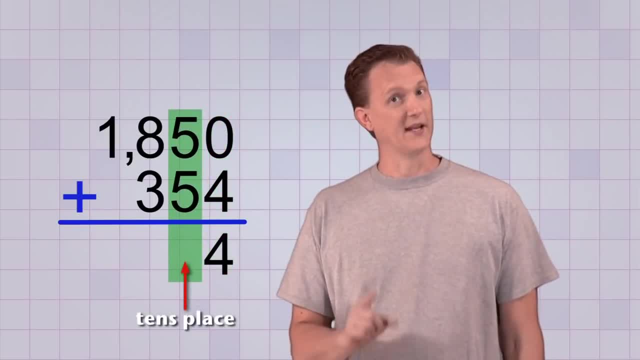 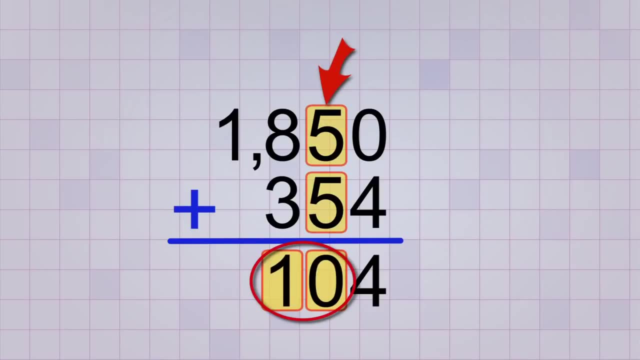 Now we move to the next place to the left, the tens place. And here comes the tricky part. If you add the digits in the tens place, five plus five, you get ten. But ten is a two digit number, so we would need to use two digits in our answer to write it. But 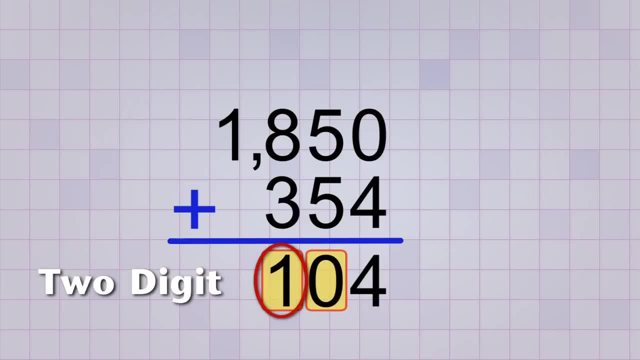 we can't leave a one in the hundreds place of our answer, because we're going to need that space when we add the hundreds place digits. That way we're going to have a number that one is going to be in the way. So what do we do? The answer is we carry the digit that we don't have room for up to. 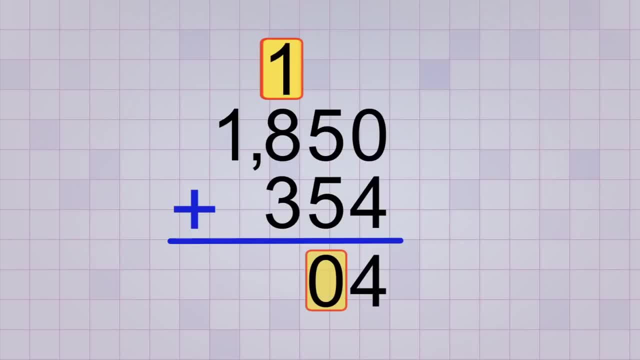 the top of the next number place column. Instead of putting it in the answers space, we put it above the other digits in our hundreds place column so that we can add it with the rest of the digits in that column. So you can see the one is going to go in the hundreds place of our answer, just not. 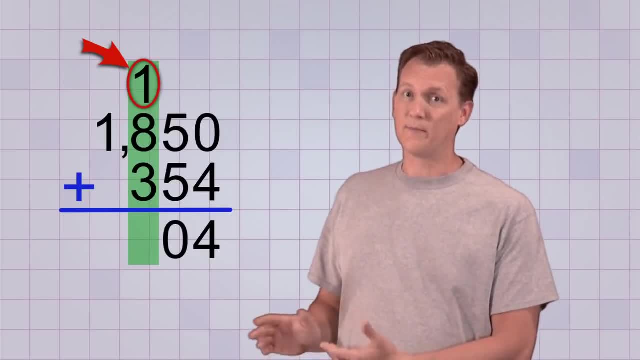 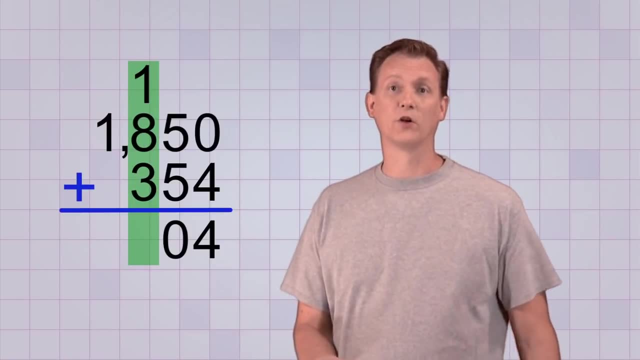 by itself. It's almost like it has to get in line so it can be added to the other digits in that column. Cool, And carrying the extra digit up to the next column you're going to add is often called regrouping, because it's really like you're moving a group of ten to the next column. 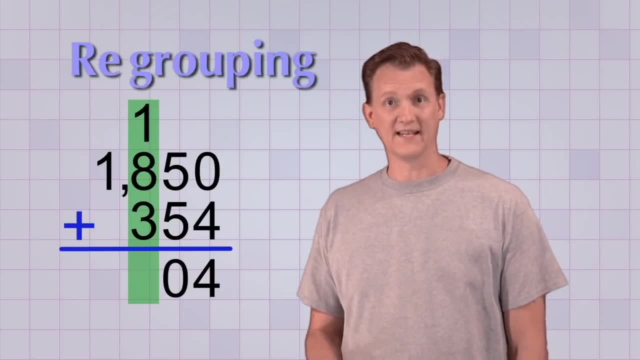 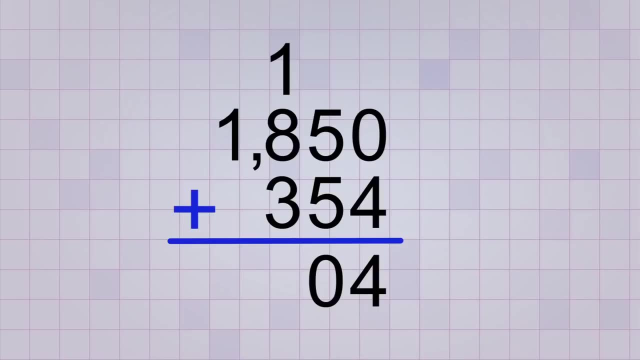 over and leaving whatever's left in the first column, In this case zero. Okay, now that we've carried that one, we can add up the digits in the hundreds place column, which means adding up three digits now: One plus eight plus three, which equals. 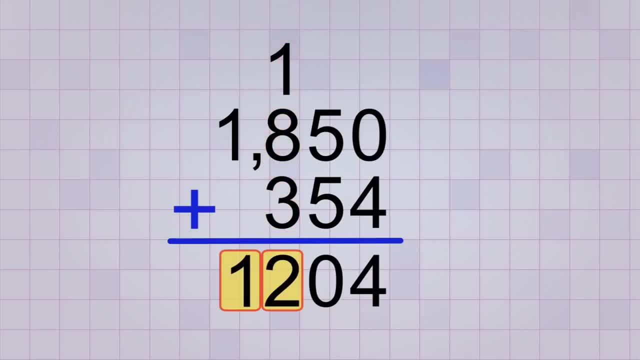 twelve. Hmm, another two digit number. Alright, it looks like we'll have to carry again because we're going to need this answer spot for the next column to the left. So we carry the one up to the top of the next column and leave our two where it is in the hundreds place of the answer. 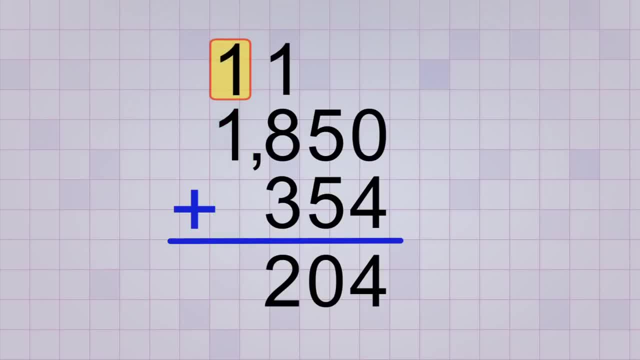 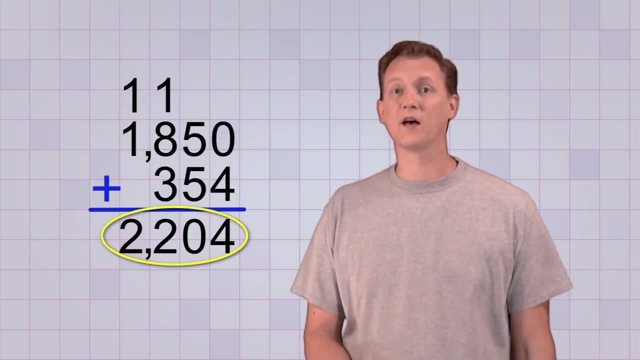 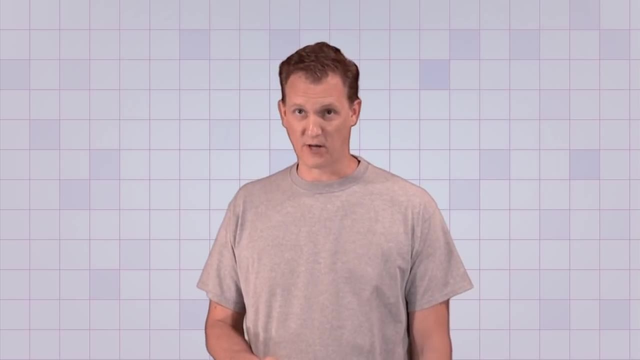 Just one more column to add up now In the thousands place we have: one plus one equals two. Okay, we've added up all our columns, so the answer to our addition problem is two thousand two hundred and four. Think you've got it so far. Let's try one more together before you do some of the exercise. 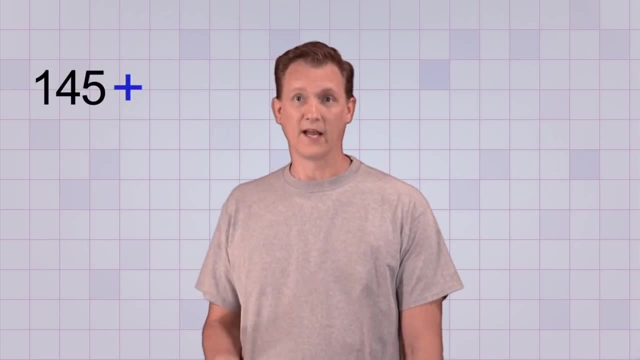 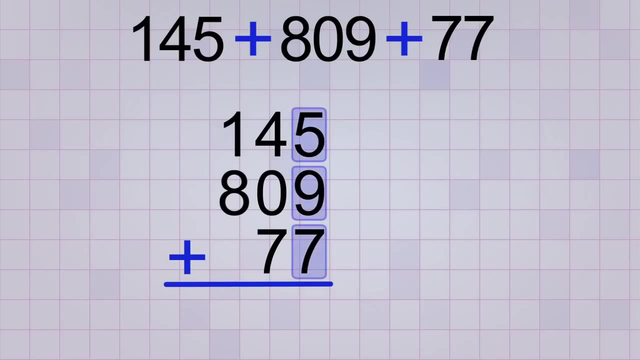 problems. Let's add up these three numbers: One, forty-five, eight, oh, nine and seventy-seven. We start the same way, stacking the numbers up and making sure all the ones places line up in a column on the right And, as always, we add up the digits in the right hand column first. Five plus nine plus. 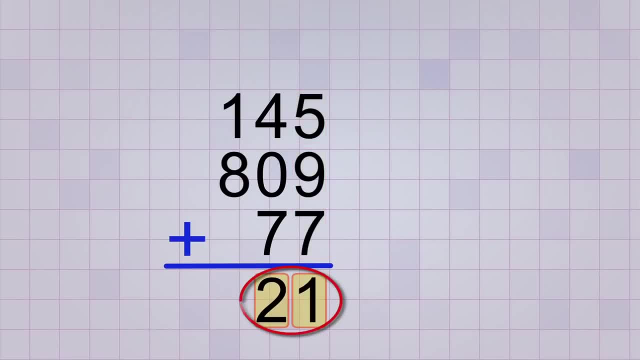 seven equals twenty-one? Because that answer is a two digit number, we need to carry the first digit to the next column, which is like moving a group of twenty over and leaving the one behind. Now we add the next column And there are four digits to add. 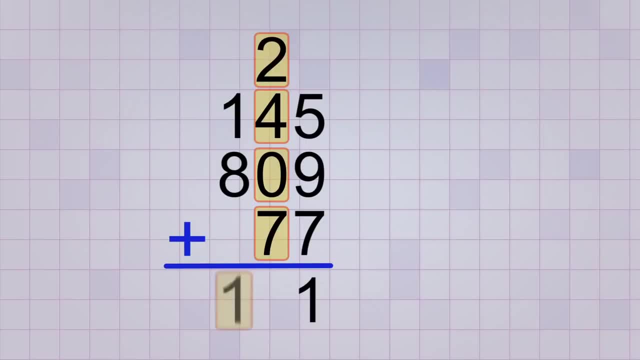 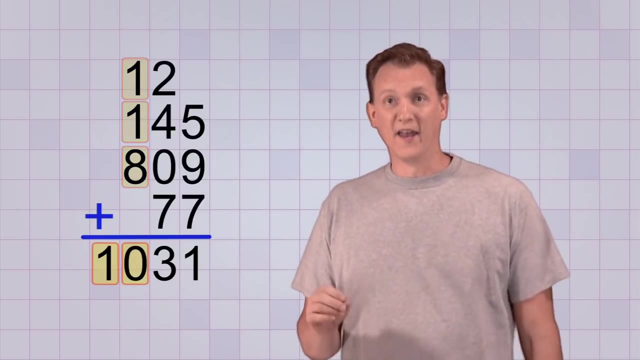 Two plus four plus zero plus seven equals thirteen. Yep, that's another two digit answer. so we carry the one and leave the three in the tens place. Last we add the hundreds place column. One plus one plus eight equals ten. Wow, another two digit number. 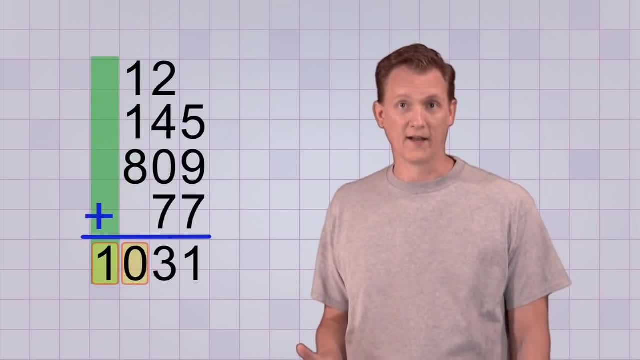 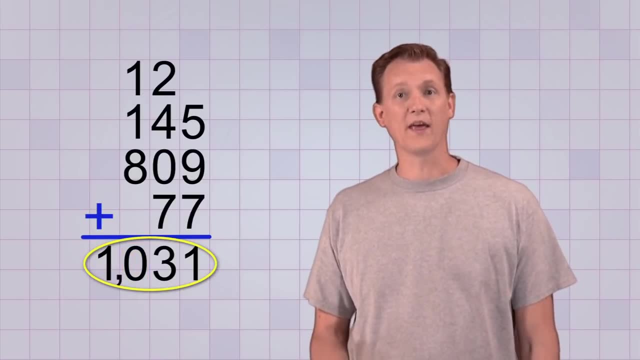 But this time we don't need to carry because there's no more columns left to add, So we won't be getting in the way of any answers by leaving both the digits in the answer like this. So our answer is one thousand and thirty-one. 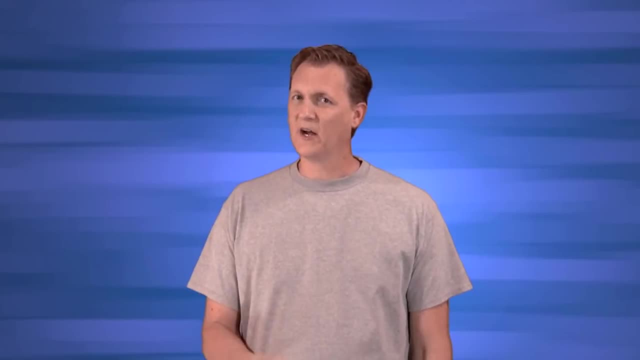 Alright, now you know how to add multi-digit numbers, But it's very important to practice so you'll remember and get good at it. So check out the printable exercises for this section. I recommend that you work a few problems each day for several days until you've got it down.